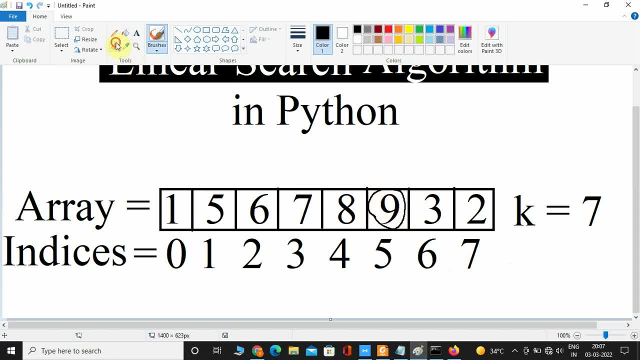 index of 9. so now the key value will be: now the key value will be 9. okay, so the now key value is 9. again, it will linearly iterate through this array. if it finds that key value- so here 9- it is going to return the index of 9. so the index of 9 is 5. what if the element 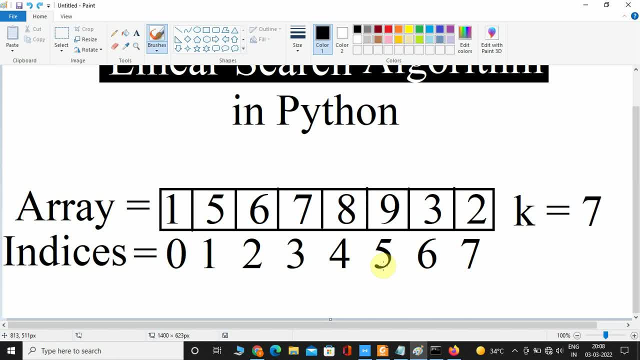 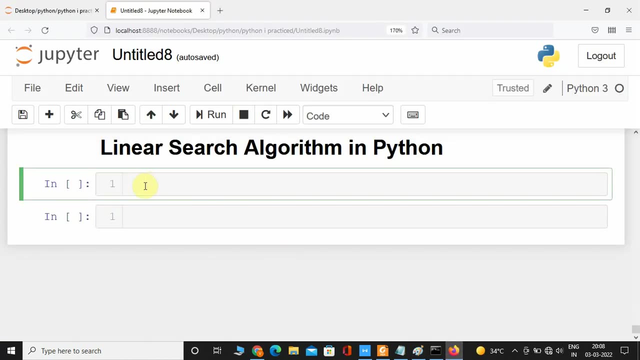 which is not present inside, inside the array, then what it will do is it will return minus 1. since my negative indexing is also supported in Python, it is not sensible to return minus 1. instead of returning minus 1, we can either return false or none. okay, so here I am in Jupyter notebook. so first things, 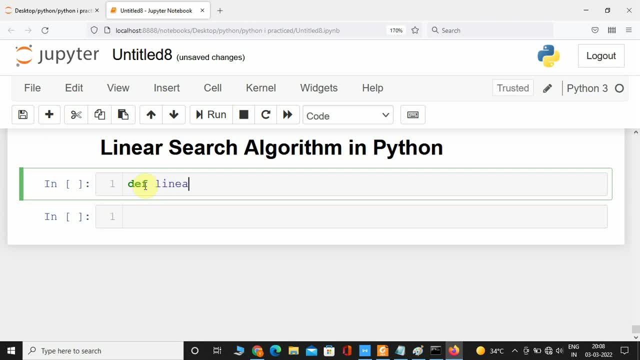 first, what I am going to do is I am going to define a function called linear search. linear search: it is going to accept 2 parameters. first parameter is list and second parameter is key. let us pass this for now. now I am going to initialize the list, which is going to have. 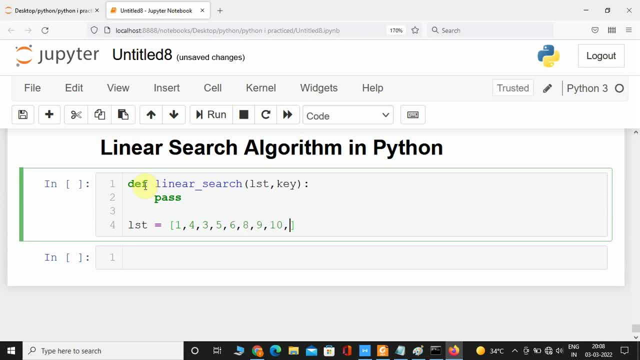 these elements, alright, and I am going to initialize key-value with 4. let us assume that we want to find the index value of 5. okay, I am going to print this now and I'm going to call this function here. okay, now that we have this driver. 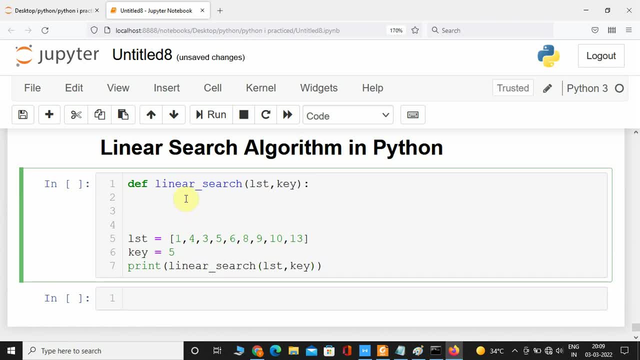 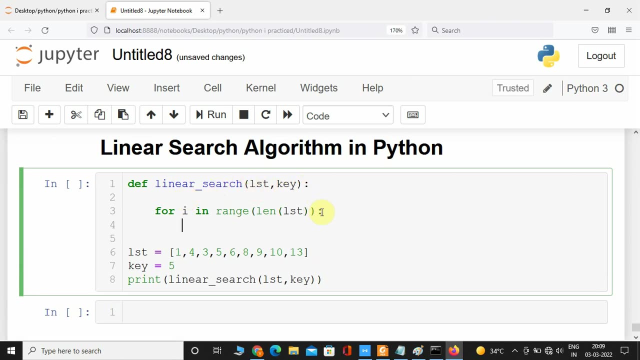 code ready, let us fill out the logic. so linear search. first things first. we need to take a for loop for iteration for I in range of length of this past list. okay, now we need to take if condition: if list of I value is equal to the key value. 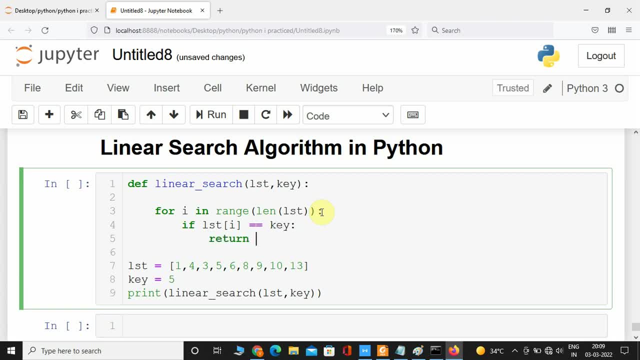 then we will return that index value. so list of that particular index value matches with our key value. then we will simply return the index of that particular key value. what if the the past key is not present inside the given list? then we will simply return false or none.